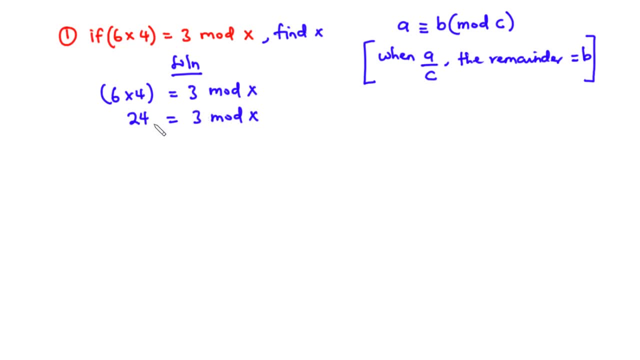 So what we are going to do is we are going to subtract 3 from 24.. So 24 minus 3 is equal to 21.. And then we are going to write down the factors of 21.. So, factors of 21,. they are 1,, 3,, 7 and then 21.. 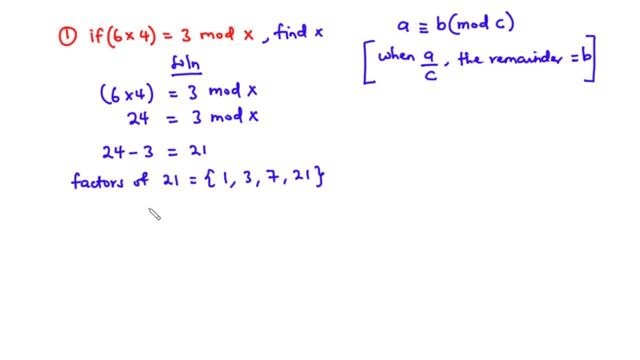 1 times 21 is 21.. 3 times 7 is 21.. Now for the factors of 21,. we are going to divide 24 by each of the factors of 21 to determine which of them will produce a remainder of 3.. 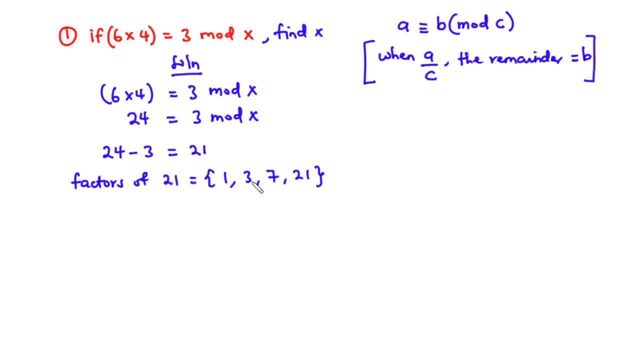 We are going to divide 24 by each of the factors of 21 to determine which of them will produce a remainder of 3.. Now the number that produces the remainder of 3 is going to be the value for x. So now let's proceed. 24 divided by 1 is equal to 24.. Remember, 0.. 24 divided by 3 is equal to 8.. Remember, 0.. 24 divided by 7 is equal to. 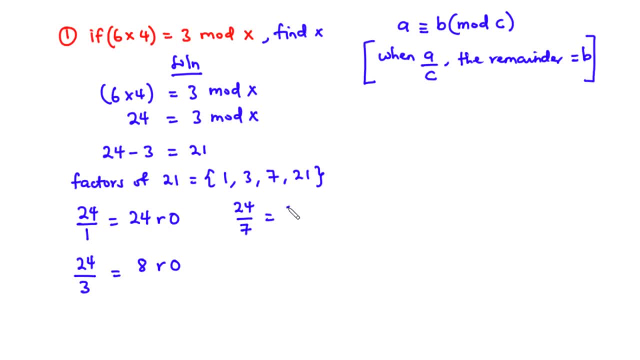 Now, 7 times 3 is 21.. So we have 3.. Remember: 24 minus 21 is 3.. So 24 divided by 7 is 3.. Remember 3.. And then 24 divided by 21.. 21 goes into 24.. Only once, Remember 3.. 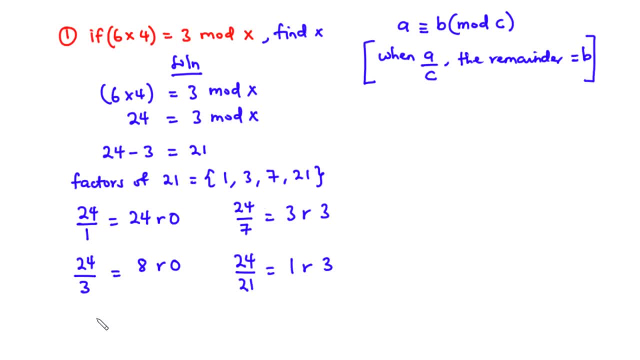 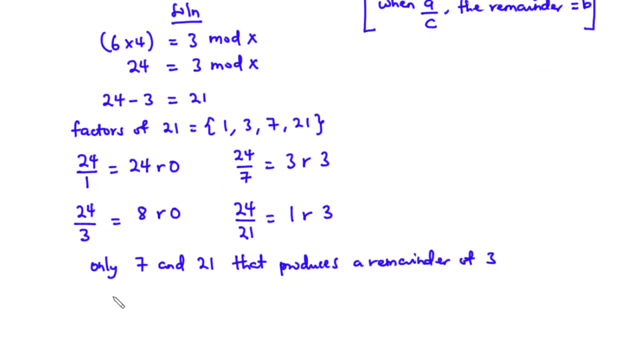 So out of the factors of 21, it is only 7 and 3. And 21, that produces a remainder of 3.. Therefore x is equal to 7 or x is equal to 21.. So, for example, 2.. 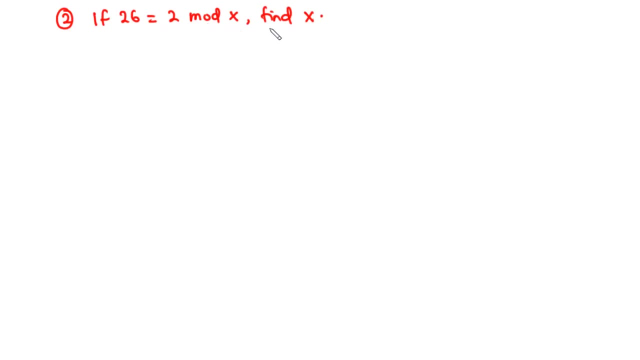 If 26 is equal to 7.. If 26 is equal to 2 modulo x, find x. If 26 is equal to 2 modulo x, find x. So, like we did in the previous example, If 26 is divided by x, then the remainder is 2.. 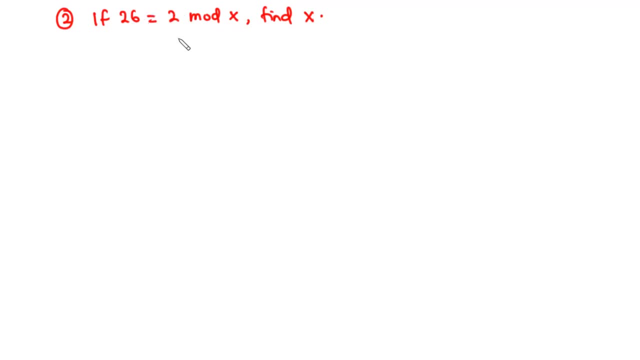 So we are going to subtract 2 from 26.. 26 equals 2 modulo x. We subtract 2.. We subtract 2 from 26 and then we have 24.. Now we are going to look out for the factors of 24.. 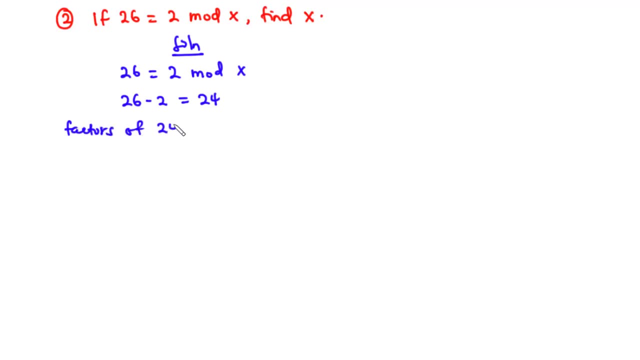 So factors of 24.. We have 1,, 2,, 3,, 4,, 6,, 8,, 12 and then 24.. 1 times 24 is 24.. 2 times 12 is 24.. 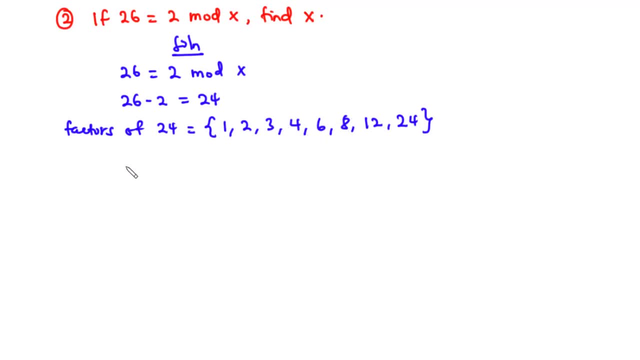 3 times 8 is 24.. 3 times 8 is 24.. 4 times 6 is 24.. So you are going to divide 26 by each of the factors of 24 to determine which of them will produce a remainder of 2.. 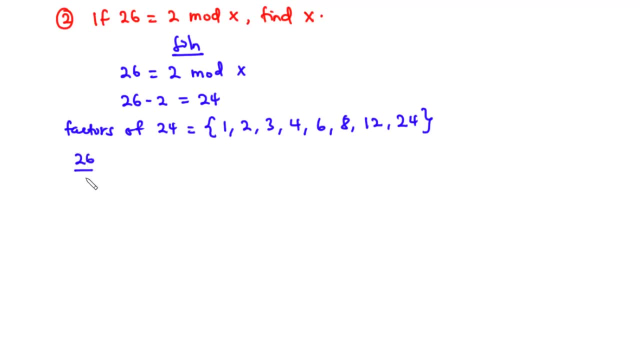 So that's what you are going to do. 26 divided by 1 is 26, remainder 0.. 26 divided by 2 is 13, remainder 0.. 26 divided by 3 is 13, remainder 0.. 26 divided by 3 is 13, remainder 0. 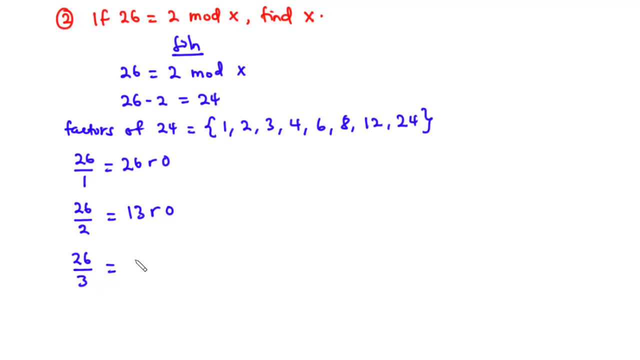 26 divided by 4 is 13, remainder 0.. 26 minus 4 is 14.. 3 times 15 is 24.. 3 times 8, which are three times 24.. رض, The слgram was equal to 32.. 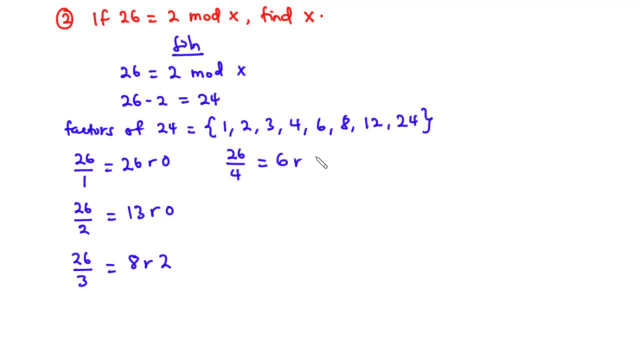 So remember that We divided- What We divided 16 by 22.. What is this? We divided it by a 3 Haitian. Now we are going to multiply 16 by 2.. 16 divided by 9? What? 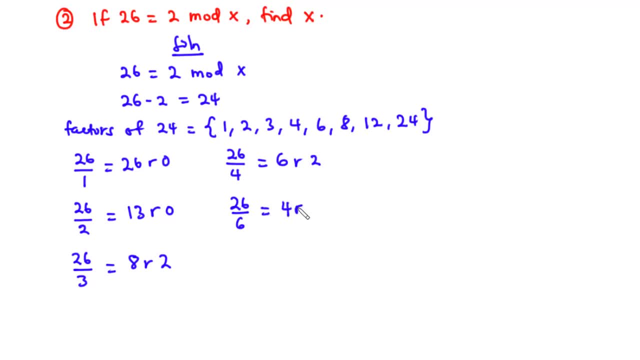 13 divided by 10? 18 hit. What times? 4 is 24, so 4 remainder 2. and then we move on to 26 divided by 8.. 8 times 3 is 24, so we have 3. 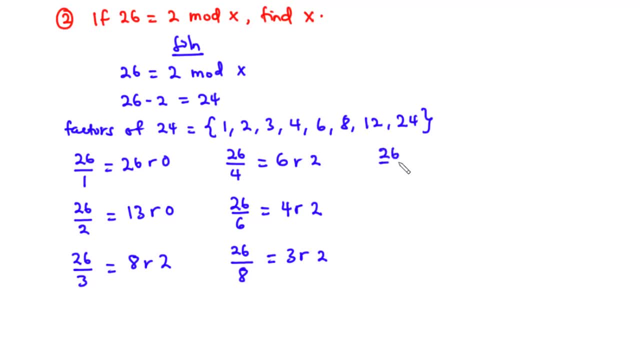 remainder 2.. Now, 26 divided by 12.. 2 times 12 is 24, so remainder 2, because 26 minus 24 is 2. and then to the last one, 26 divided by 24.. 24 goes into 26 once, and then remainder 2.. 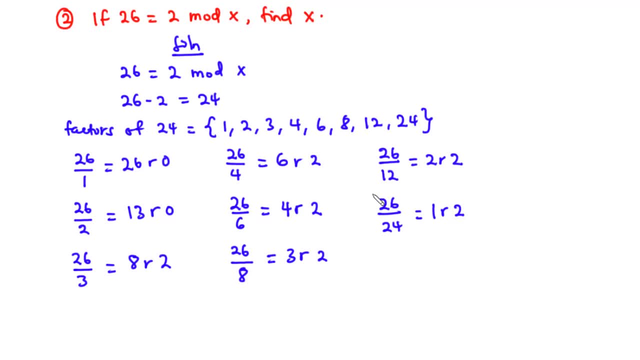 So 3,, 4,, 6,, 8,, 12 and then 24, after dividing 26 produces a remainder of 2.. Therefore x is equal to 3,, 4,, 6,, 8,, 12 or 24.. 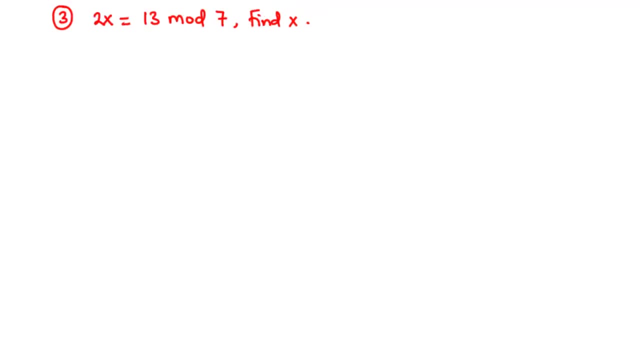 Now let's solve question 3.. You realize that question 3 is slightly different from the other two examples that we've solved so far. Here we have 2x equals 13 mod 7, and then we are asked to find the value of x. Now we said that when you have an expression like this, 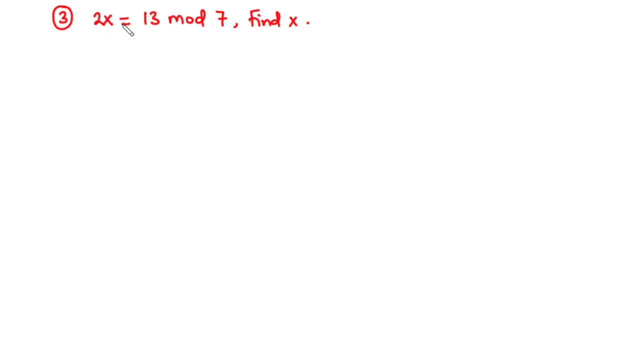 then what this primarily means is that when 2x is divided by 7, the remainder is 13.. So what you are going to do is we are going to find the multiples of 7, that, when you add to 13 or subtract from 13, you are going to get a value that is divisible by 2.. 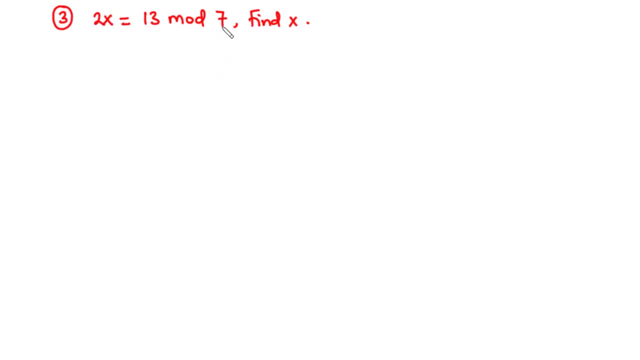 I'm going to repeat this again. You are going to find the multiples of 7 that when you add to 13 or subtract from 13, you are going to get a value that is divisible by 2.. Now let's write down the multiples of 7.. 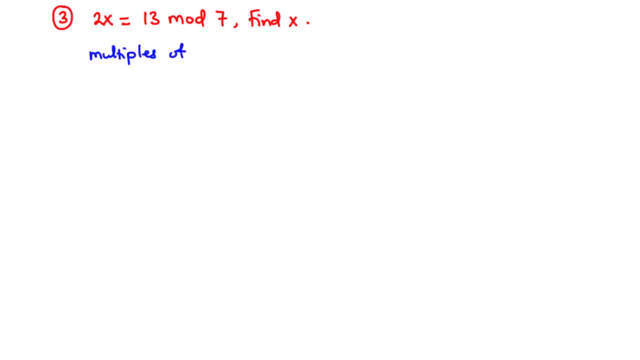 So the multiples of 7, we have 7,, 14,, 21 and so on and so forth. 7 times 1 is 7,, 7 times 2 is 14,, 7 times 3 is 21.. Now let's start off with 7.. 7 plus 13 is 20.. Is 20 divisible by 2?? Yes, 2 goes. into 20 10 times. Now let's start off with 7.. 7 plus 13 is 20.. Is 20 divisible by 2?? Yes, 2 goes into 20 10 times. Now let's start off with 7.. 7 plus 13 is 20.. Is 20 divisible by 2? Yes, 2 goes into 20 10 times. 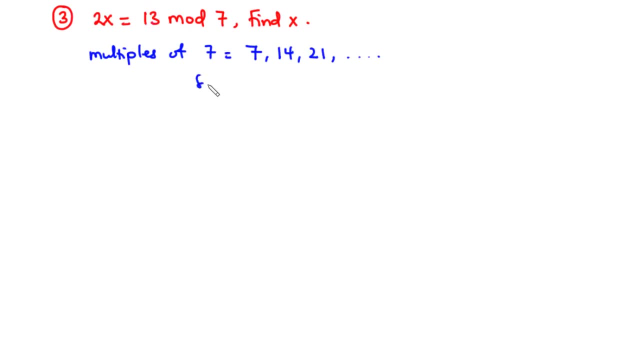 So let's add 7 to 13.. First of all let's rewrite the question: 2x equals 13, mode 7.. Now let's add 7 to 13. So that's 2x equals 13 plus 7. 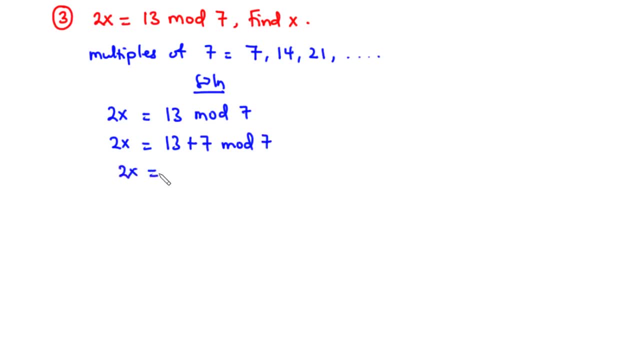 mode 7. And this is equal to 2x equals 20 mode 7.. Now we are going to divide through by 2 to get the value of x, So x will be equal to 2. goes here once into 20, 10 times. So we have x equals 10 mode 7.. Now this is correct. However, 10 is greater than. 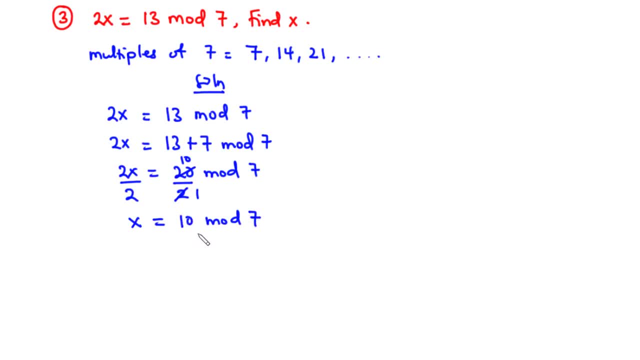 7.. Now 10 divided by 7 is 1 remainder 3.. Therefore, x is equal to 3, mode 7.. So this is the value of x. Now we are going to use a second approach. Now, instead of adding 7 to 13,, we are going to subtract 7 from 13.. So this becomes: 2x equals 13 minus 7. 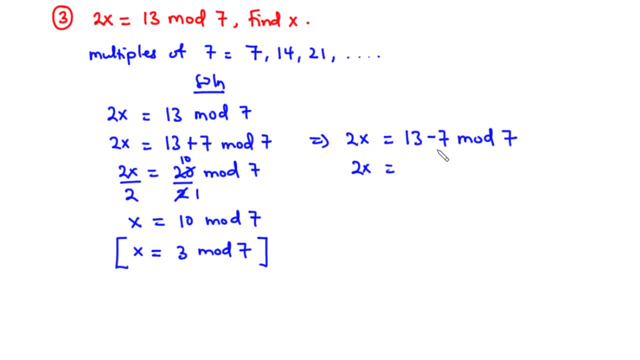 mode 7.. 13 minus 7 is 6.. So we have 6 mode 7.. You divide 3 by 2.. And then you have x to be equal to 3 mode 7.. So you can either choose to add multiples of the modulo to this number. 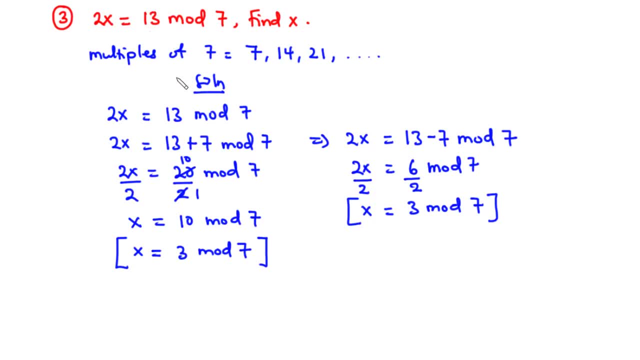 or subtract multiples of the modulo from this number. whichever way you do it, If you do it rightly, then you are going to get the final answer to be the same. Now let's solve one more example on this. So for question 4, 25x equals 15 modulo 29.. Find the value of x. 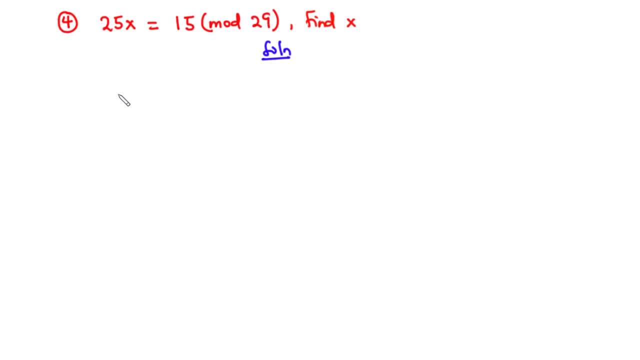 So we are going to approach this question the same way we did for question number 3.. First of all, let's write down the multiples of 29.. so for multiples of 29, we have 29. 29 times 2 is 58, 29 times 3 is 87, and so on and so forth. 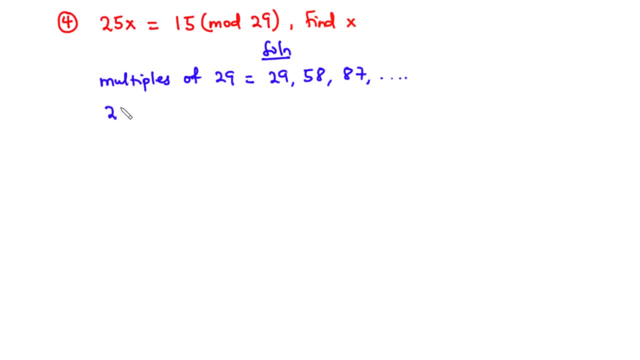 now let's rewrite the question. we have: 25 x equals 15 modulo 29. now 25 and then 15 are multiples of 5. so we can divide through by 5 to reduce the equation. so this becomes 5 x equals 3 modulo 29. at this point we are going to add or subtract. 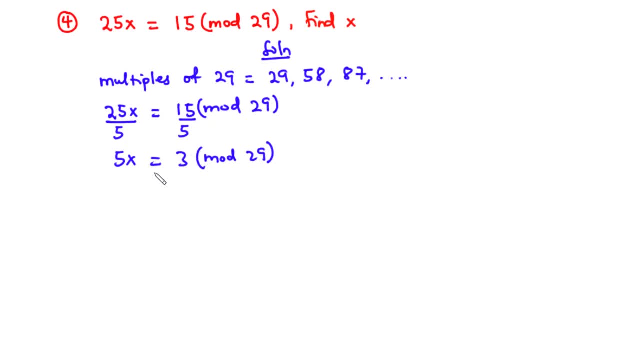 multiples of 29 from 3 and then to determine which of them will be divisible by 5, so that we can find the value of 5 of x. so let's start with addition now. 3 plus 29 is 32. 32 is not divisible by 5. let's move on to 58. 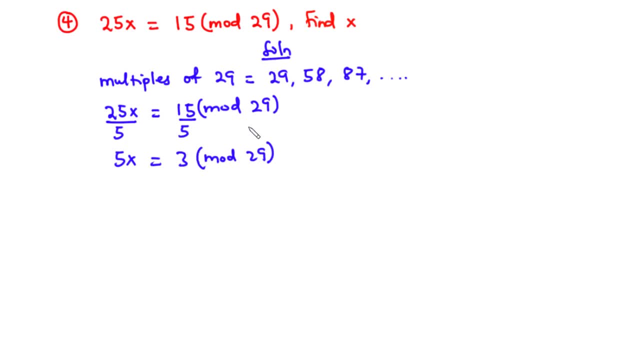 3 plus 8 is 61, which is also not divisible by 5. now let's look at the reverse. we are going to subtract multiples of 29 from 3. 3 minus 29 is negative 26, which is not divisible by 5. 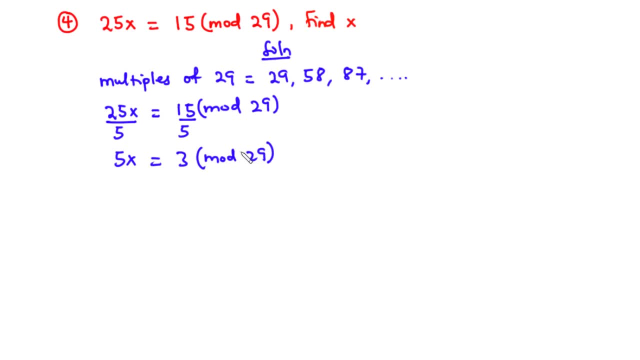 3 minus 58 is negative 55 and that is divisible by 5, so we are going to subtract 58 from 3, so that's going to be 5 x equals 3 minus 58 modulo 29. 3 minus 58 is negative 55. 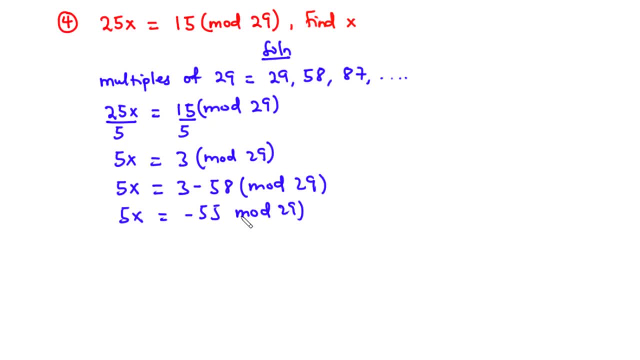 and then we divide through by 5, so we have: x equals negative 11 modulo 29. now this time we have a negative number, so we need to convert this to a positive number, less than 29. in doing so, we are going to add 29 to negative 11 until we get a positive number. 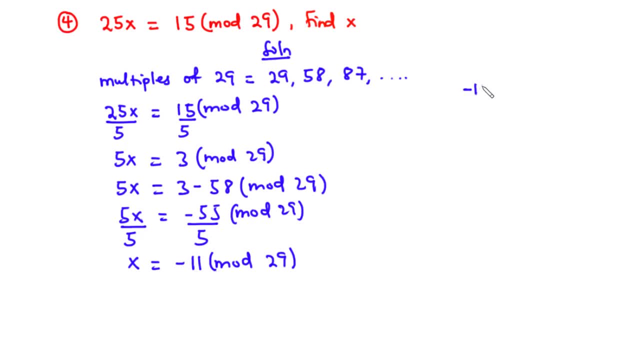 less than 29. negative 11 plus 29 is equal to negative 29, so we have a negative number. less than 29 equal to 18, 18 is a positive number and then less than 29, so it follows that x is equal to 18 modulo 29. this is the value of x.